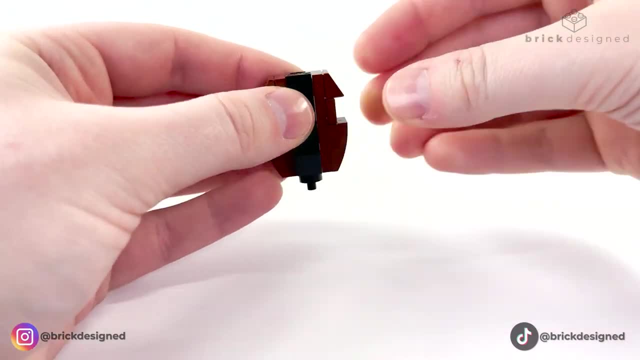 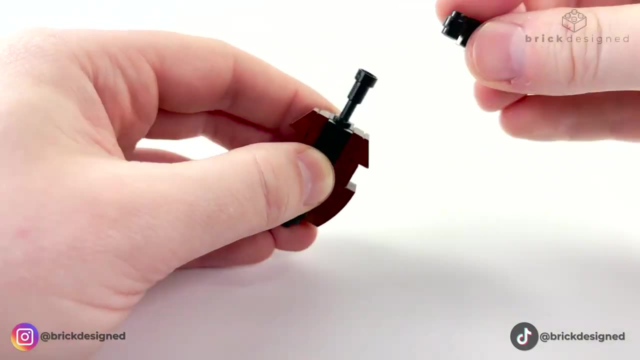 was actually requested by one of my subscribers and it inspired this video and this theme, so I hope I did it justice. When I'm building, I really try to focus on accuracy. I want to provide a build that is as detailed as possible and also to scale with the minifigure. With these instruments, I 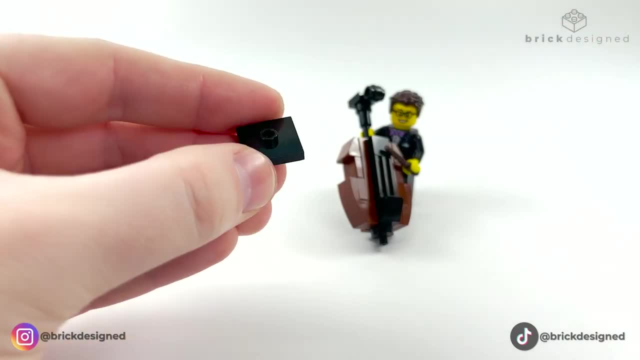 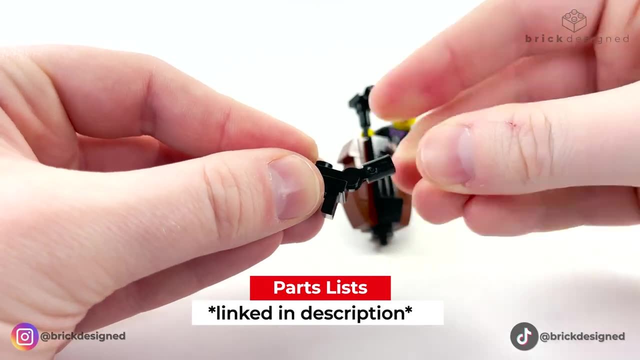 really focused on the shapes and the layout. I really wanted to do them right, so I hope you guys enjoy. I love how they turned out and I did include parts lists for each instrument in the description below And, as always, smash that like button for me and please consider subscribing. 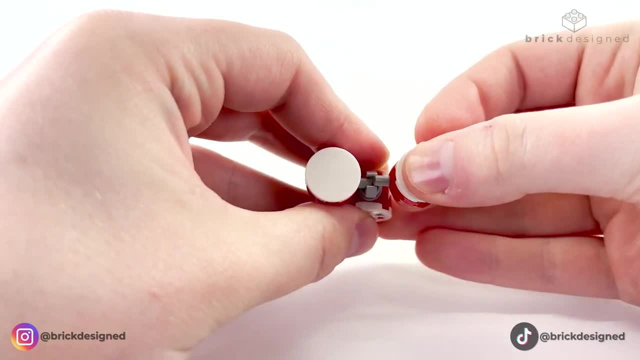 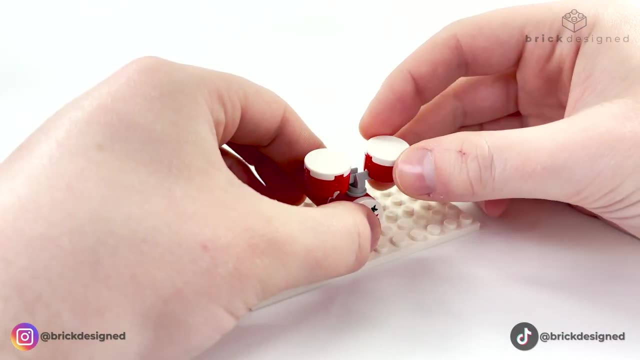 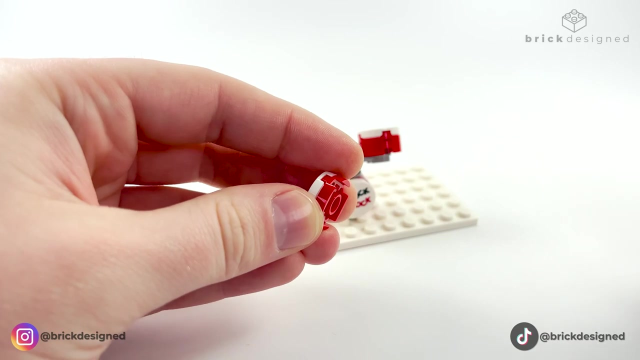 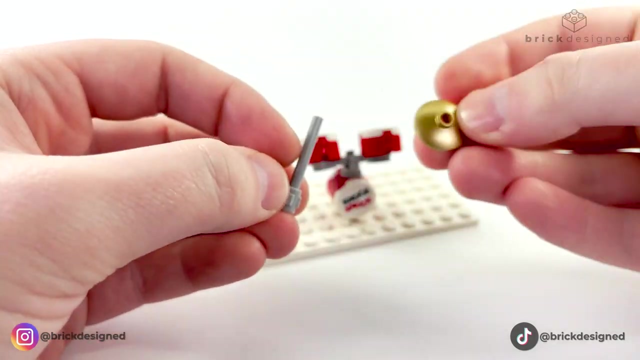 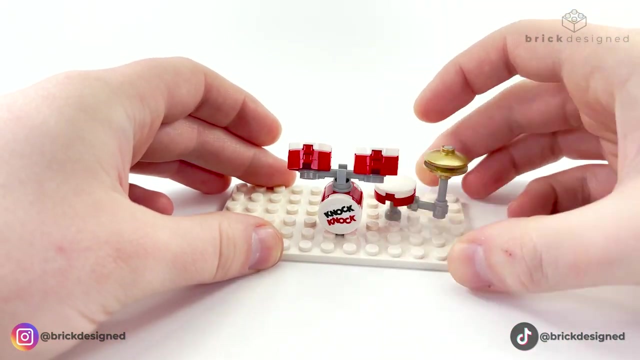 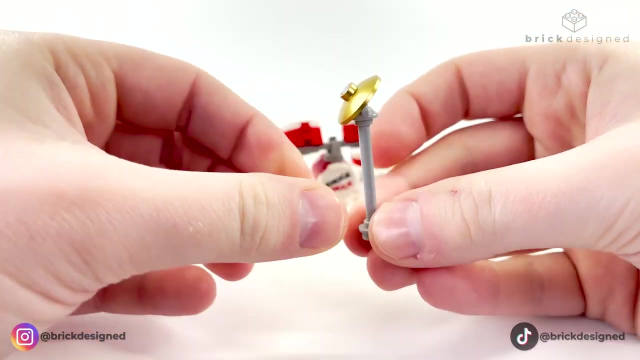 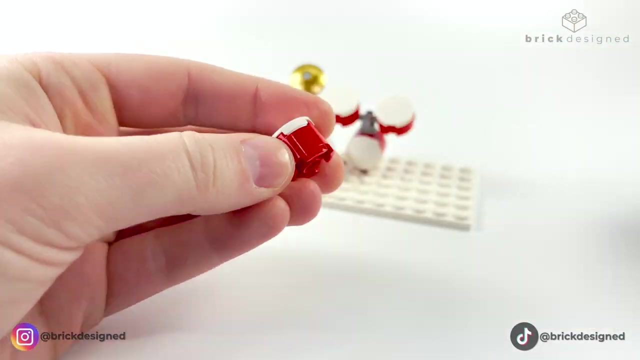 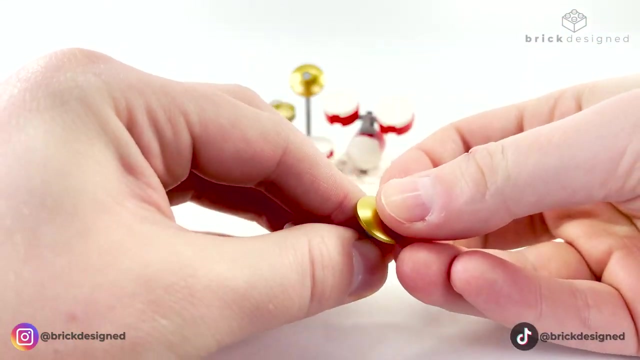 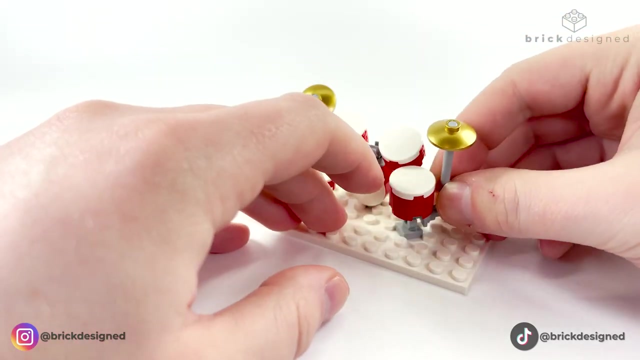 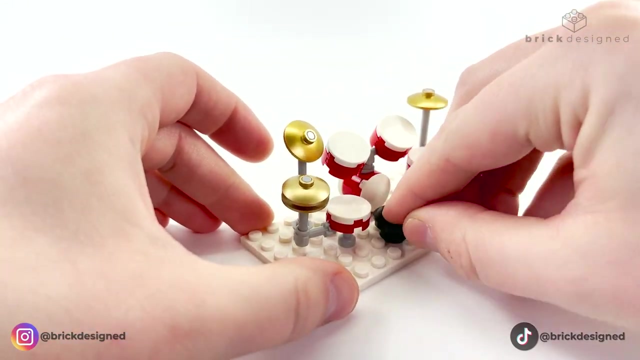 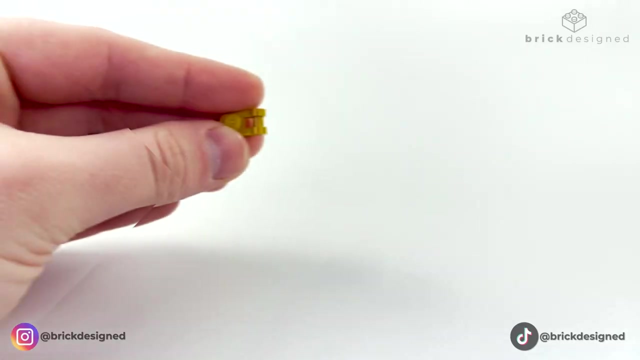 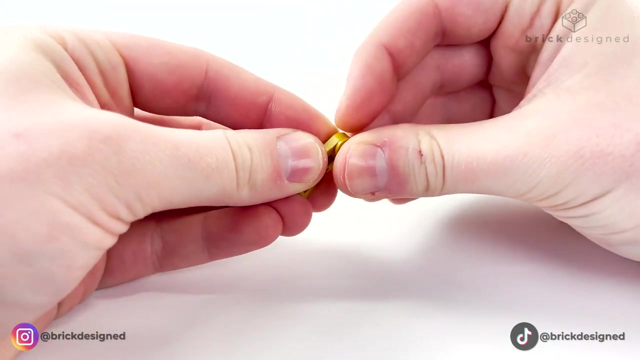 Thank you so much for watching and I'll see you guys in the next video. Thank you for watching and I'll see you guys in the next video. So when you're building this harp, just be aware it is a little flimsy, just because of all the 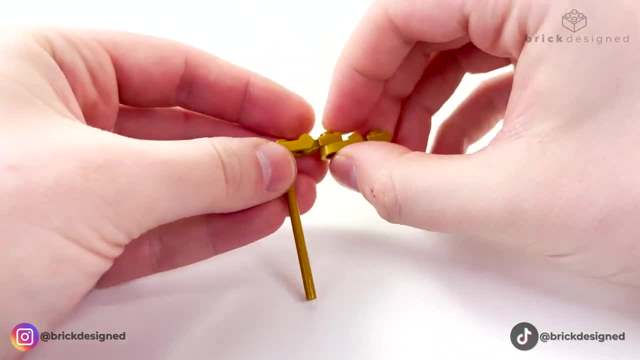 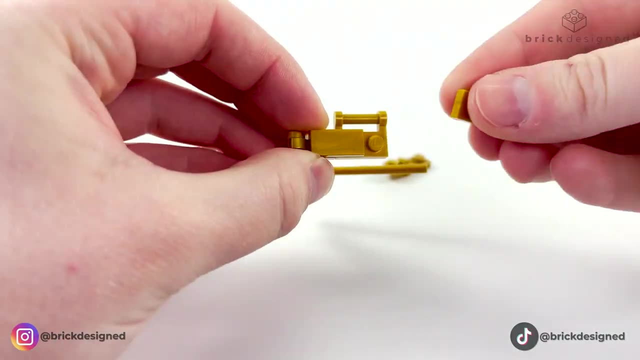 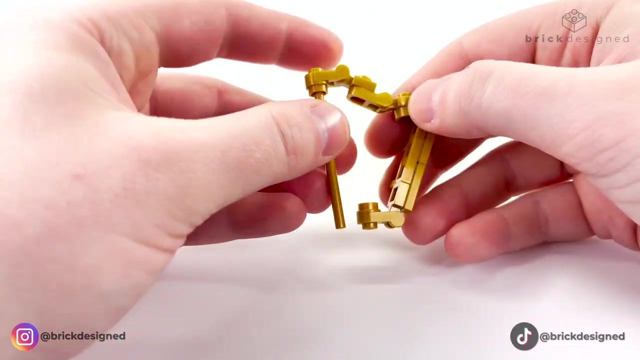 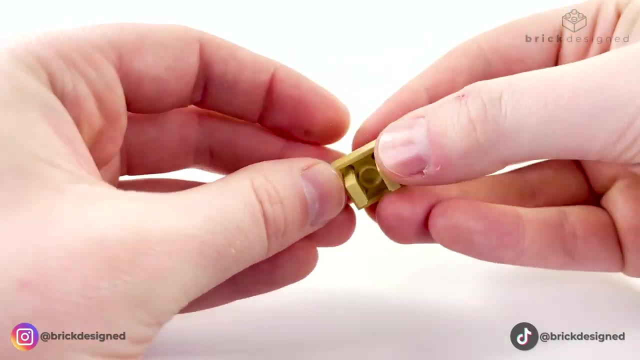 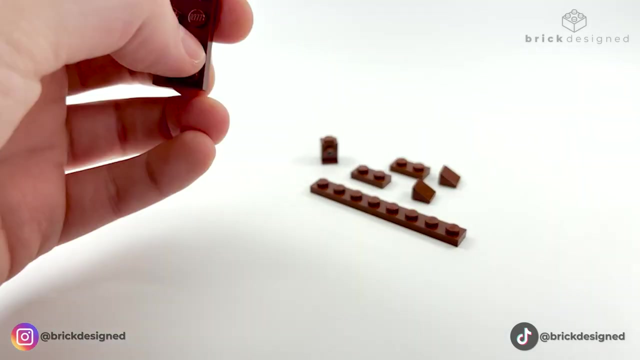 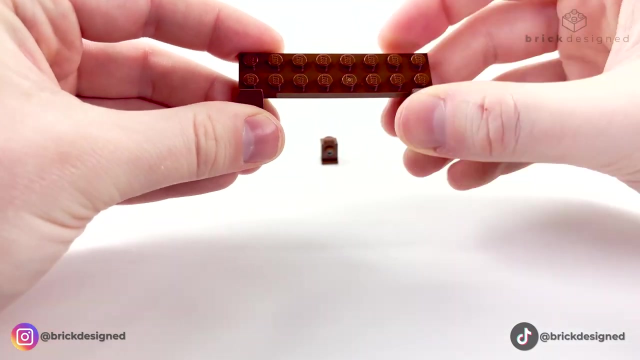 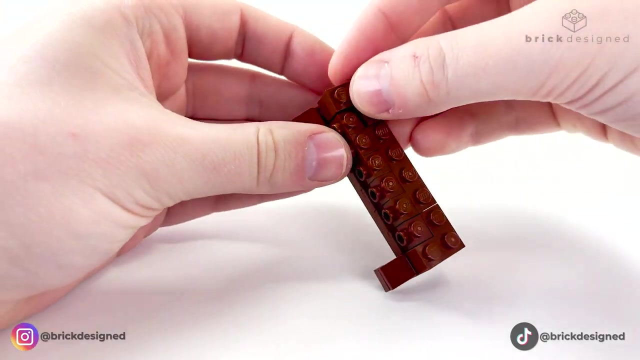 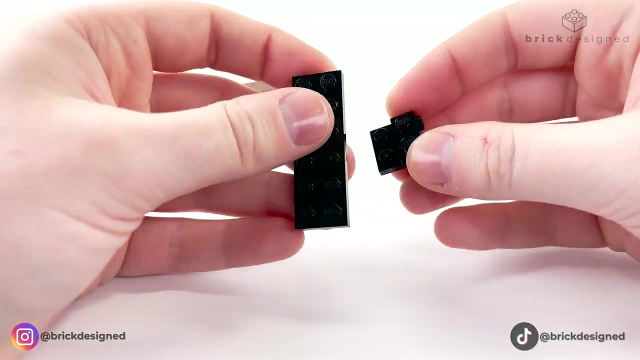 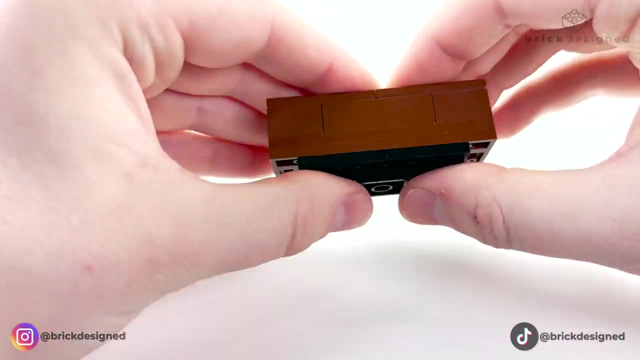 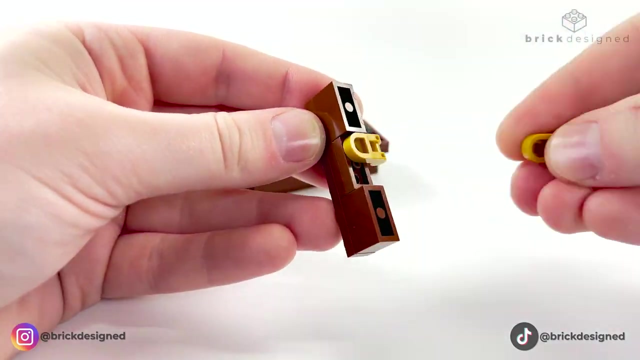 different angles and the connections that are going on with these pieces. So just play around with it and it should all come together pretty easily. Thank you so much for watching and I'll see you guys in the next video. Thank you for watching and I'll see you guys in the next video. 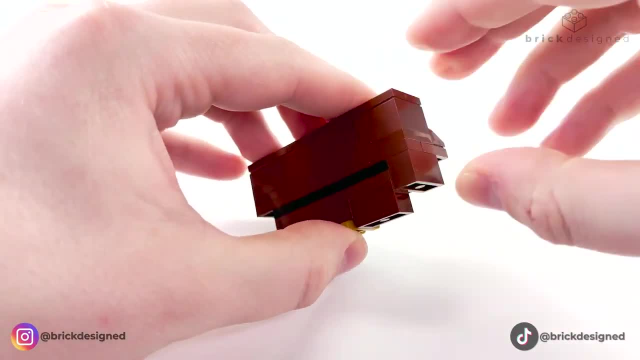 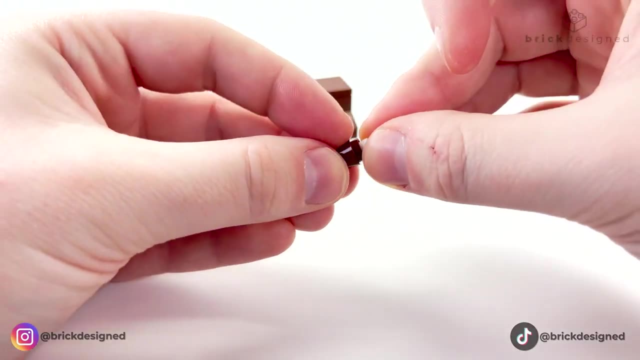 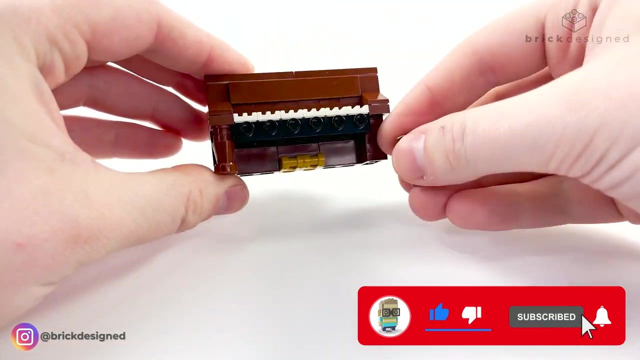 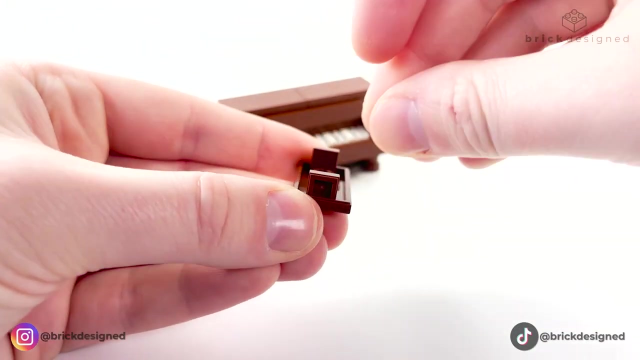 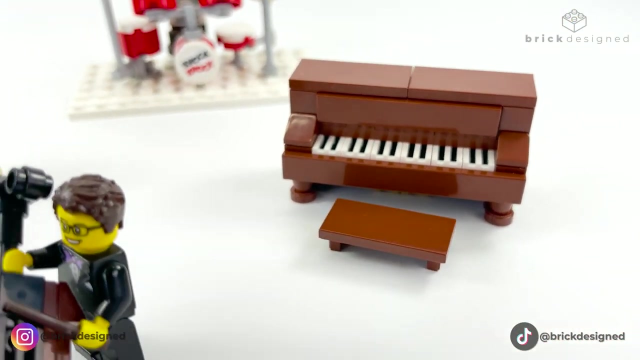 Thank you for watching and I'll see you guys in the next video. Thank you guys, so much for watching. I hope you enjoyed. You can always see my other tutorials on Instagram and TikTok at brickdesigned, And let me know in the comments down below which instrument you like the best or what you'd like. to see me build next And I'll see you guys in the next video. 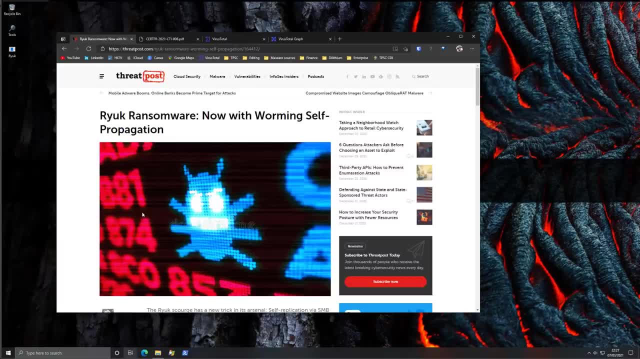 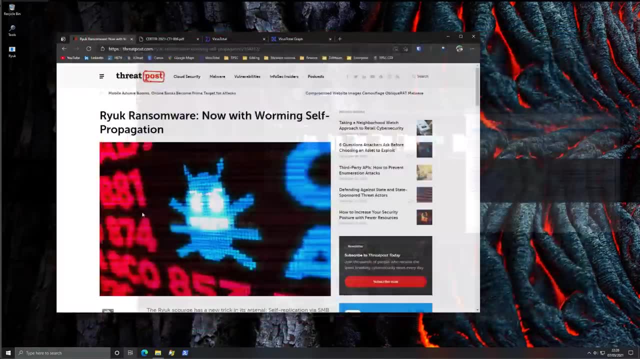 Hello and welcome to the PCSecurity channel. Today we'll be taking a look at Ryuk ransomware. As usual, we'll do a live analysis, run the ransomware on a test VM, see what happens and give you the best advice to defend against it. 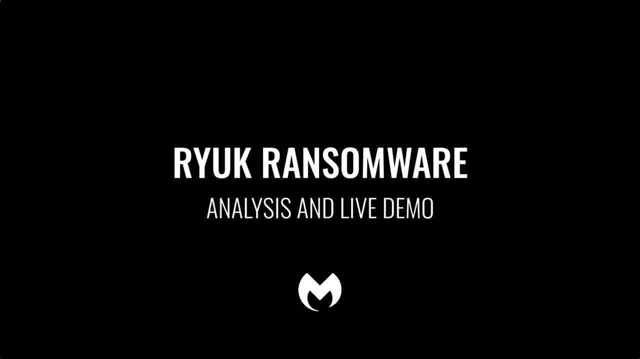 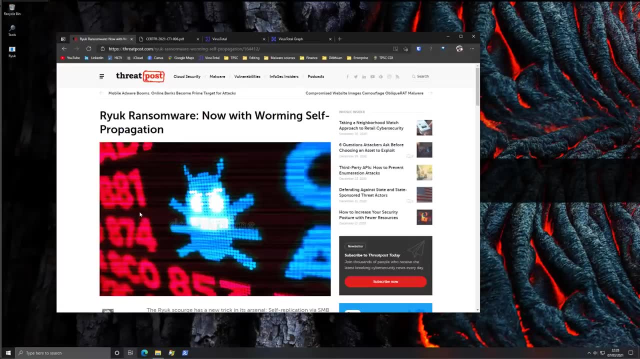 This video is brought to you by Malwarebytes Privacy. Check them out using the link in the description. Alright, so why am I talking about Ryuk right now, given that this is a ransomware that's been around for about two years now? There are several reasons for it, First of all, 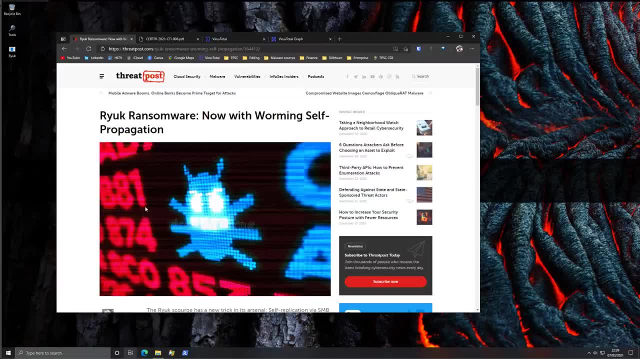 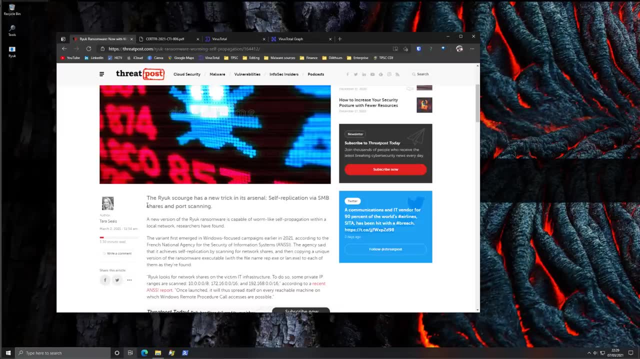 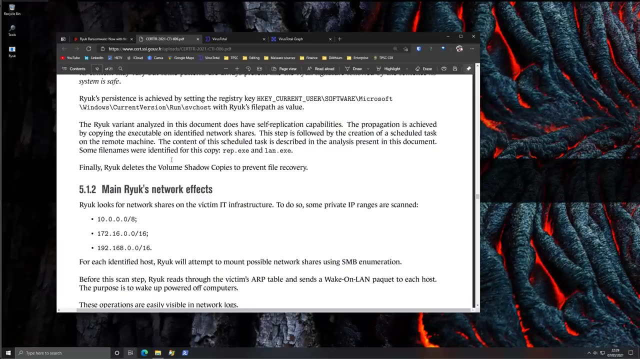 there's a brand new variant, and this one has a lot of worm capabilities, including self-propagation via network shares. If you are someone who is managing the network of a company, you should take note of some of the IP ranges that it's going to attack, So 10.0.0,, 172.16, 192.168.. 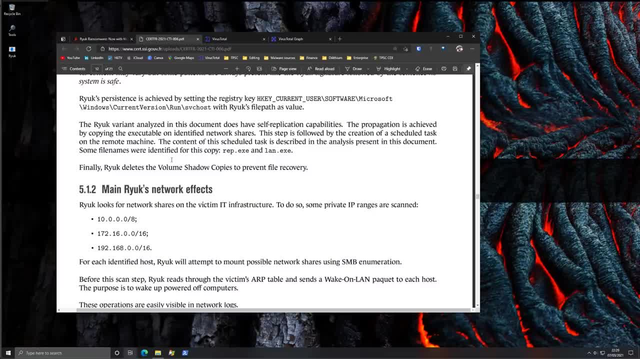 These are very common local ranges of IP addresses, And what Ryuk is going to do is it's going to look for any network drives system locations that can be found in these address ranges and promptly start to encrypt them. One of the things 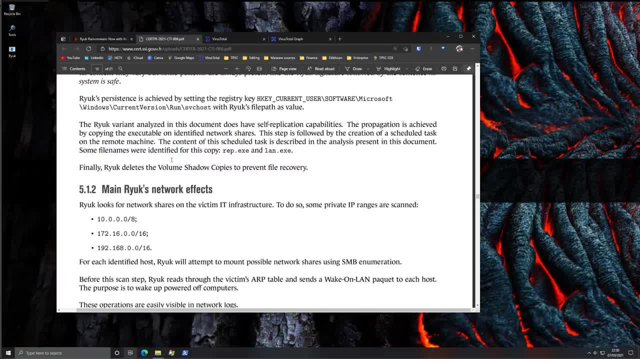 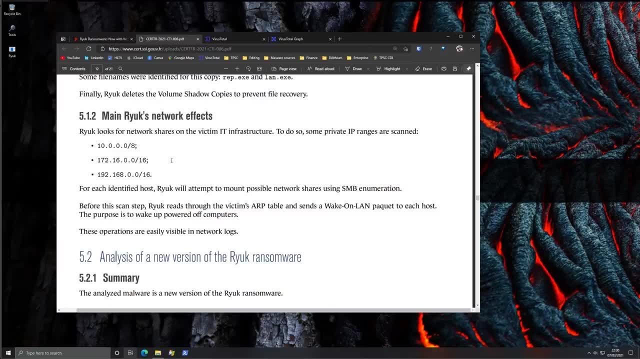